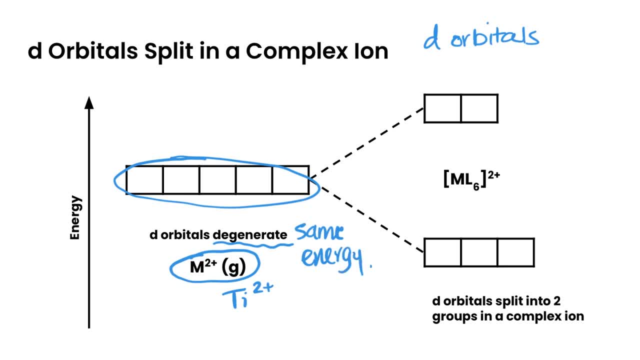 However, if you now take that metal ion, so if we took a titanium ion and we put it in water, we're going to have the formation of a complex ion. So a complex ion where we take the metal and we surround it by, say, for example, six different ligands, then the d orbitals are no. 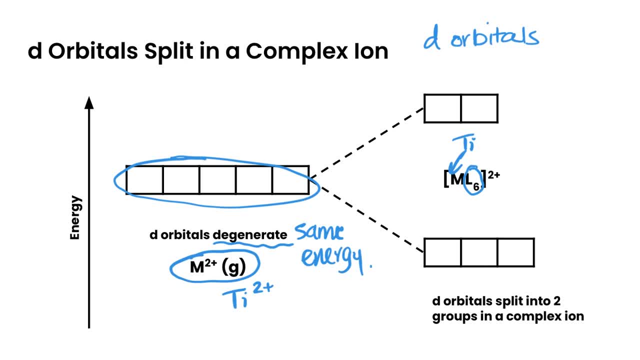 longer degenerate. So we're going to have a complex ion where we take the metal and we surround it by, say, for example, six different ligands. then the d orbitals are no longer degenerate And they actually split into two groups. There for the octahedral shape, three of the groups. 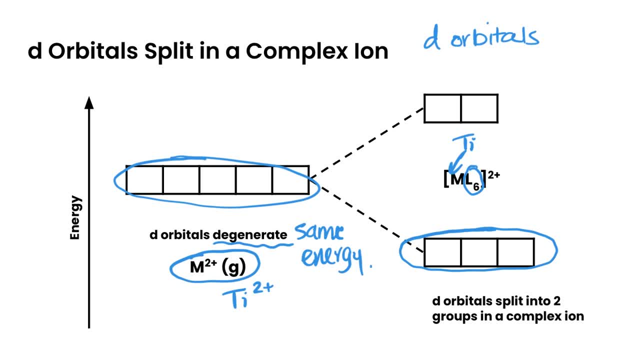 are lower energy and then two of the groups are higher energy. So you end up getting a splitting pattern for the d orbitals themselves, And so this diagram shows the splitting pattern for an octahedral complex ion. If you had, for example, a tetrahedral complex ion, you would get a different splitting pattern. 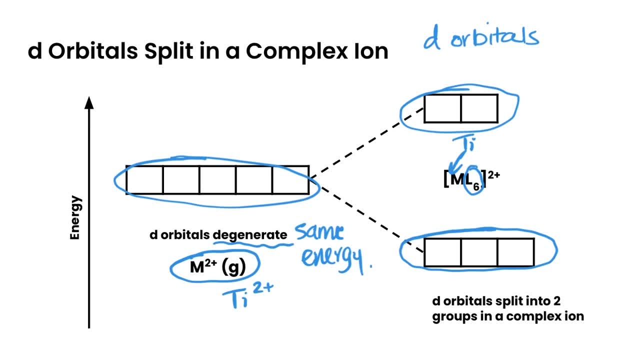 But we're just going to kind of look at this splitting pattern because this is complicated enough. And so the reason why we get that splitting pattern in the d orbitals is because it's caused by repulsion between the electrons in the metal ion d orbitals and the lone pairs of 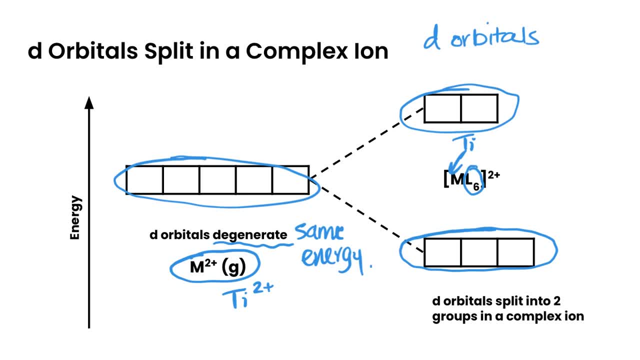 electrons in the metal ion d orbitals, And so the reason why we get that splitting pattern in the distance is because we're not going to have a split spectrum of electrons on a single ligand, And so for poleostomy the two d orbitals are going to be less than one, and we have 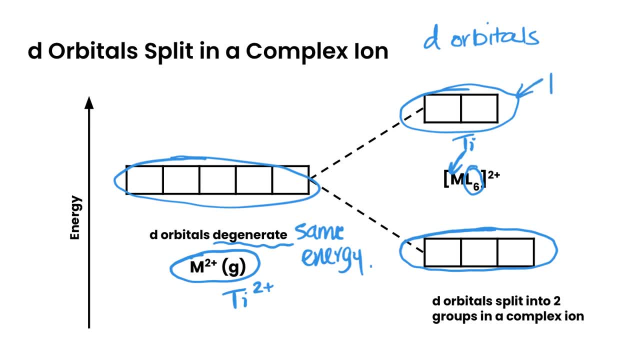 a better deal of energy because we had less than one and we have less than one pectron on the ligands. So in the octahedral shape two of the d orbitals are going to point directly at the lone pair. So these ones are the d orbitals pointing directly. 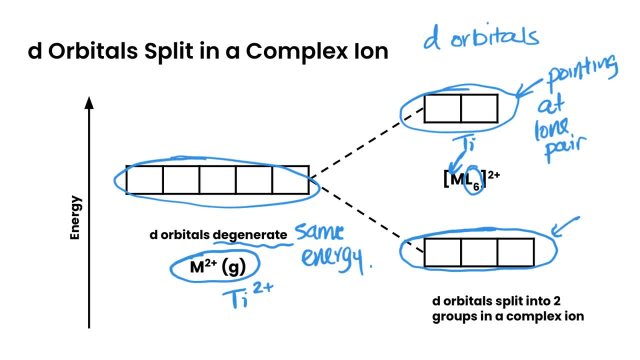 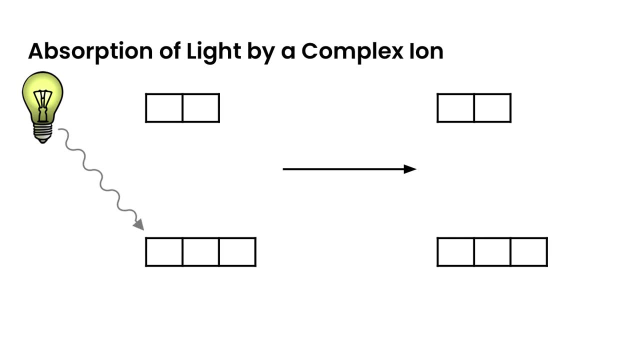 So these ones are the d orbitals pointing directly, So they're pointing at the lone pair, so they become higher energy, the lower energy. Okay, and this is where our splitting patterns come from. Now, when we take a transition metal ion complex, so a complex ion- and we have an electron in one, 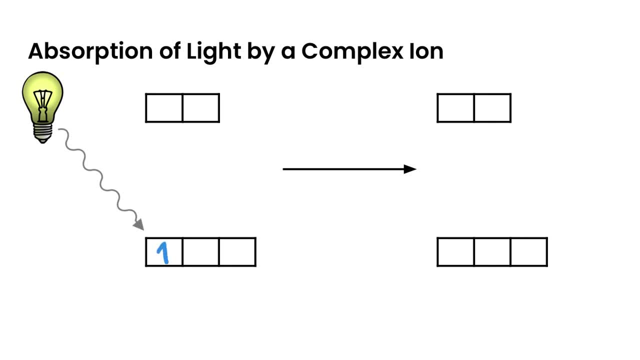 of these lower d orbitals and we shine white light on it, we can actually promote that electron. it will absorb the energy and it'll get promoted up to one of the higher energy orbitals. So this one here is up here and we are absorbing the light energy. 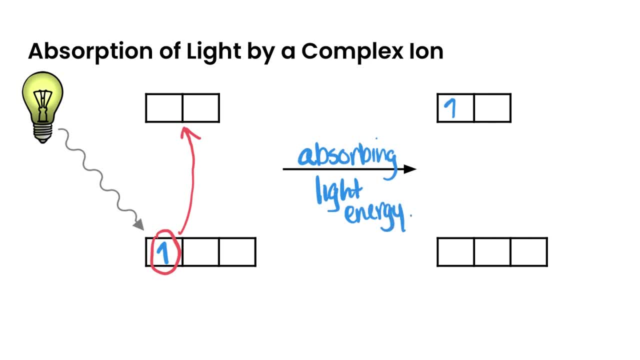 And depending on how much the d orbitals have split, it's going to require differing amounts of energy or different frequencies or wavelengths of light in order to absorb and promote that electron to the higher set of d orbitals. It's kind of similar to what we saw when we looked at 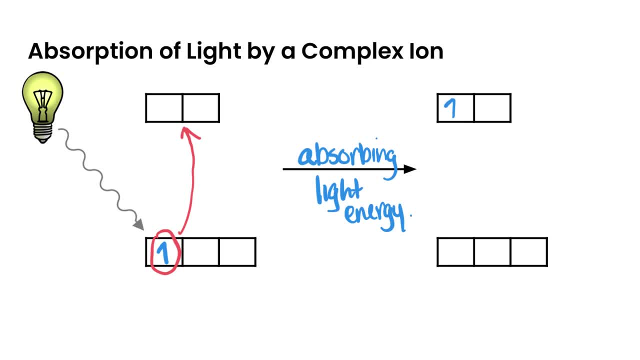 the absorption of light, and electrons being promoted up to a higher set of d orbitals. So the same sort of thing is happening here, except the electrons are being promoted within the d orbitals themselves. It's just now. we have this splitting pattern. So 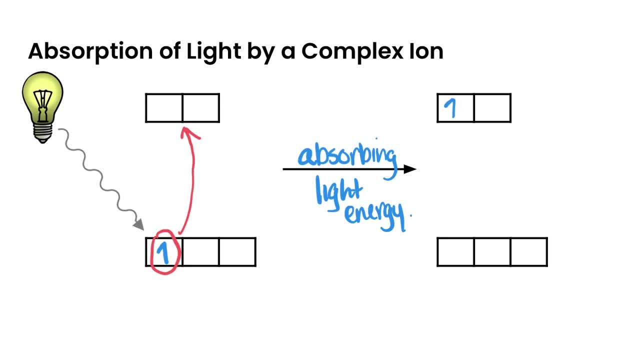 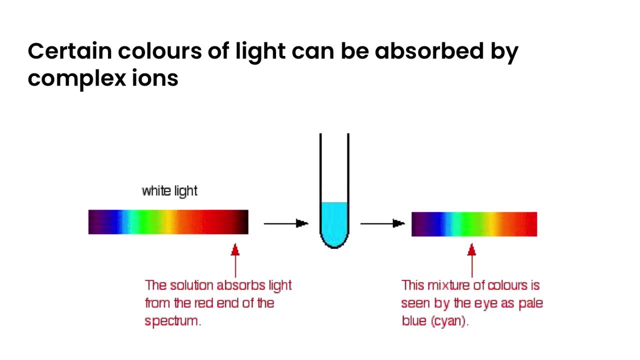 they're being going from the lower set into the higher set of d orbitals. So when we shine light on complex ions, certain colors of light can be absorbed by the complex ions. So when we shine light on complex ions, certain colors of light can be absorbed by the. 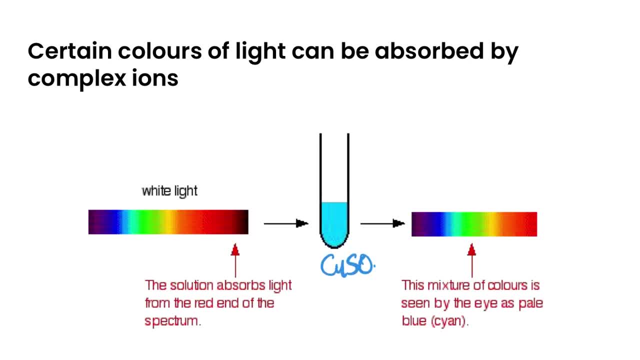 ftenic金. in other words, through the d orbitalenson, through the other, reconstructing succes. so Honeycomb hina, where we saw a Yellowstone shine for the whole time. If, for example, we take a solution of copper sulfate and we pass white light through this. 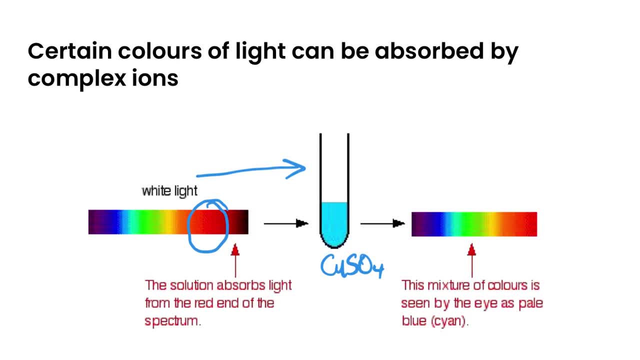 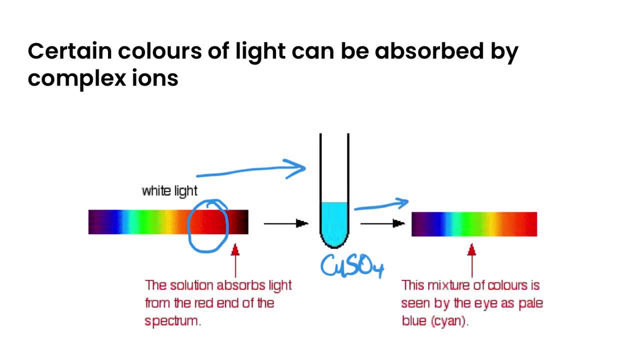 So when that orange end of the spectrum is absorbed it's going to promote an electron from the lower set ofd orbitals to the higher, 6101, 00 knows electrorente from the lower set of d orbital. Waterman is absorbed And then the light coming out of this solution is everything but that orange sort of end of the. 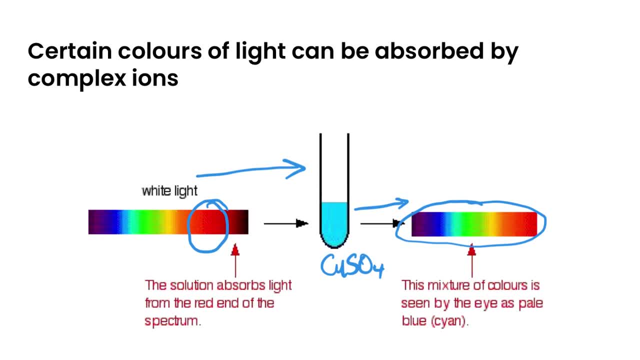 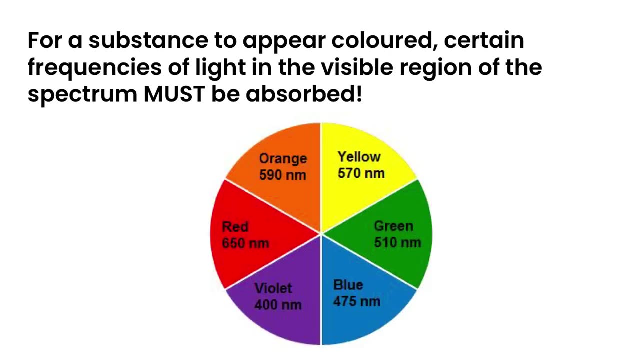 spectrum. So it results in a bluish kind of color, which is the complementary color to orange, which is what we're seeing. So we're seeing everything but the light that is being absorbed. Now for a substance to appear colored, certain frequencies of light in the visible range of the 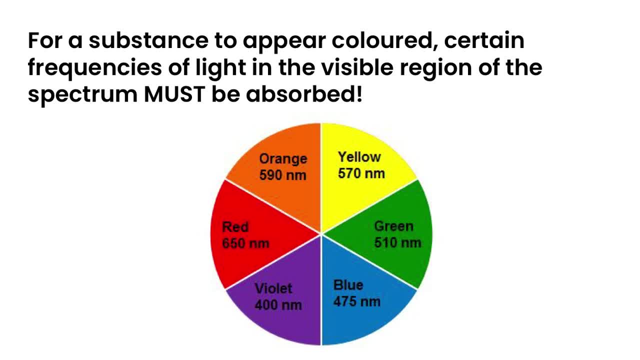 spectrum has to be absorbed And we can use a color wheel to figure out. if we know the color of the substance, we can figure out the color that's being absorbed, or vice versa. So, for example, the copper sulfate solution: we can use the copper sulfate solution to figure out the color. 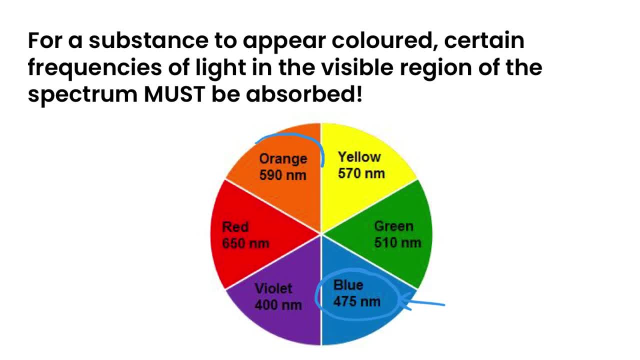 of the solution, And that's because the orange or the complementary color to it is being absorbed. So if we had, say, a solution that appeared green, then the red light is being absorbed. Or if we had something appearing yellow, the violet light is being absorbed, And so that's. 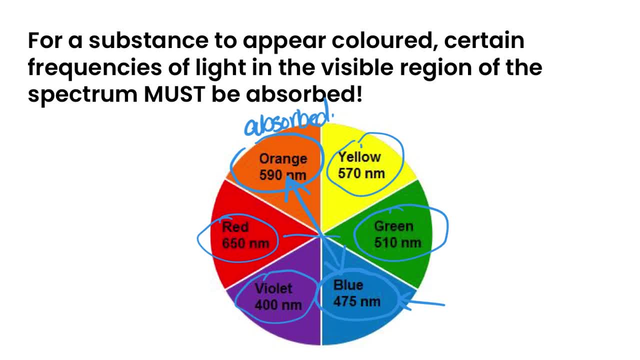 telling you information about what particular color it is, And then we can use a color wheel to figure out what the color is being absorbed. And then it also tells you the wavelength, which then gives you information about the frequency as well as the energy that's associated with that. 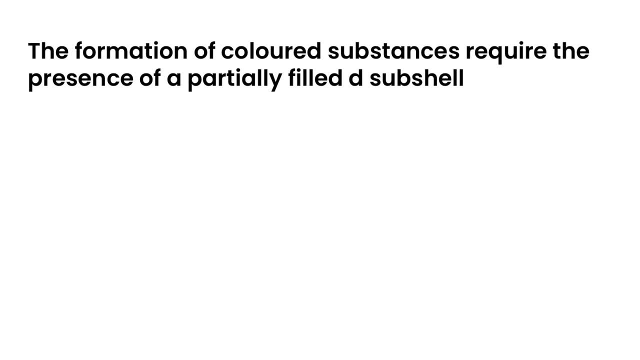 absorption. Now, finally, the one thing we do need to point out here is that the formation of colored substances require that there is a partially filled D subshell present. So if the D subshell is fully filled, or if it's fully empty, there are no electrons that can be. 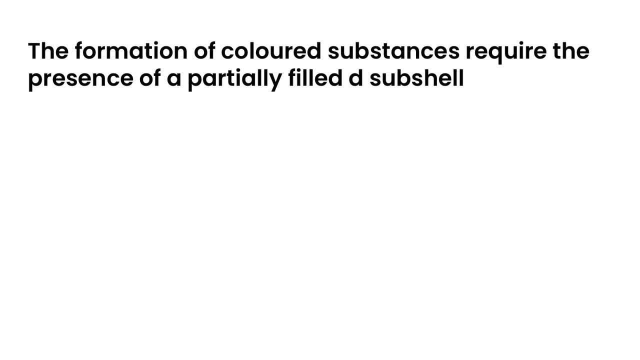 promoted up to the higher set of orbitals, which means that you don't get this effect. So they essentially remain colorless. So a couple of examples here: if we have a scandium 3+- remember, scandium by itself is 4s2, 3d1.. So it would have none of those electrons, but it would.